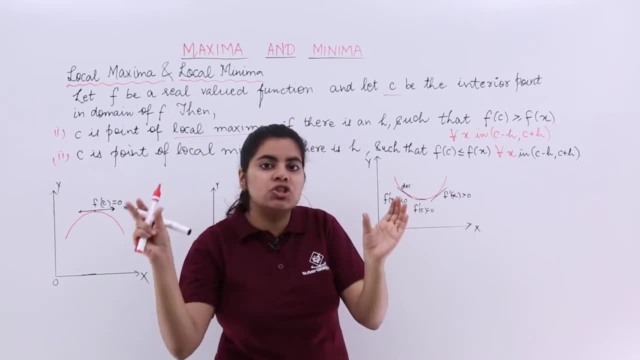 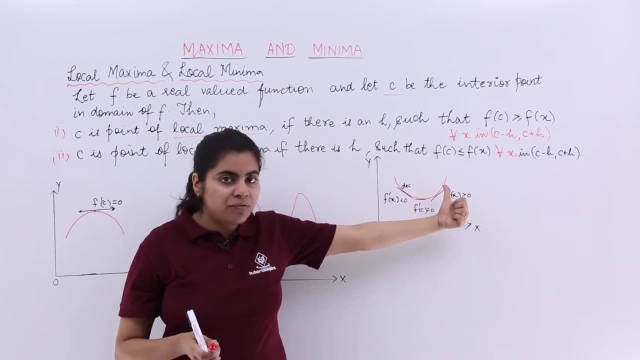 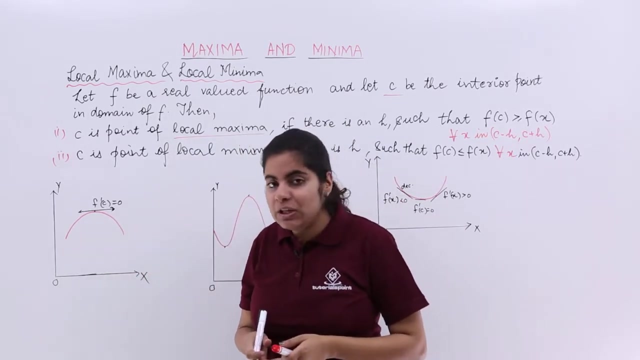 And we are talking about a restricted domain- c minus h to c plus h, c minus h to c plus h- where h is greater than 0.. So let's talk about this graph later and let's talk about this graph now. Now you have, this is the curve given to you, and you can see that the curve is such that 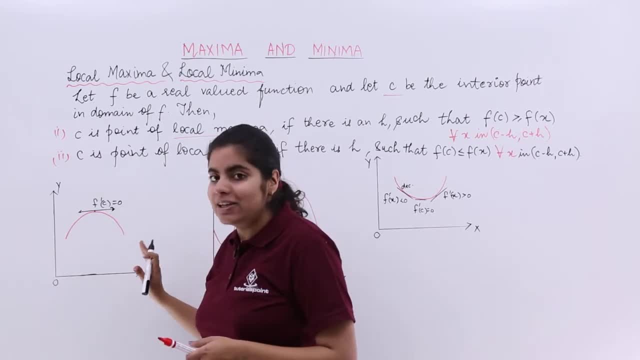 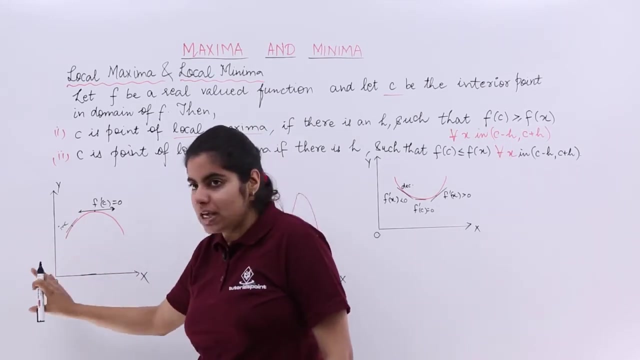 from the 0. that means towards the positive direction of the x axis. you start moving. you start moving and you find a point here and you see that if you draw a tangent it will be going upwards. That means the graph is increasing over here. So if it is c minus h case, and this is c plus h case, you see the graph increases. 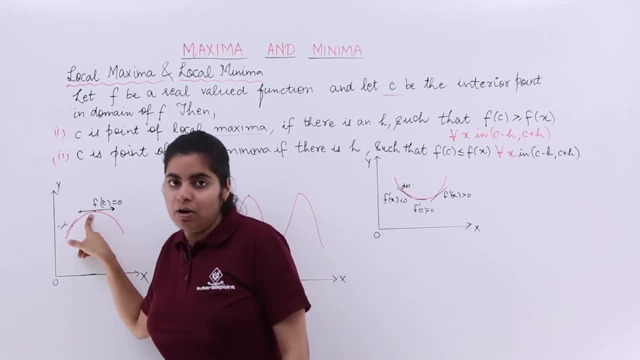 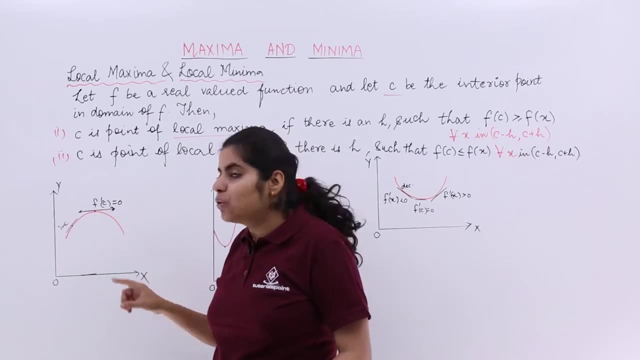 Then a point comes, when it is the peak of the graph, wherein the graph attains the maximum value. So it is the maximum value, So it is the maximum value, So it is the maximum value. And then again it goes down. and here, if I have to draw a tangent, I can find it goes down. 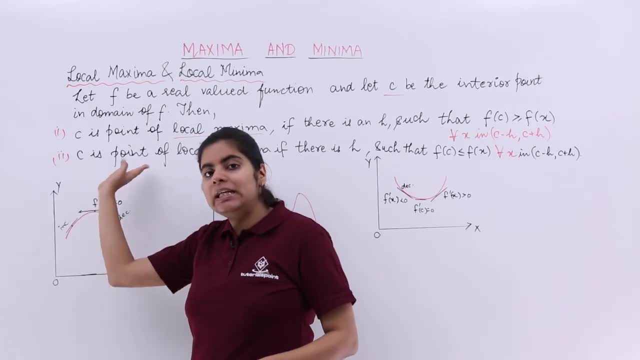 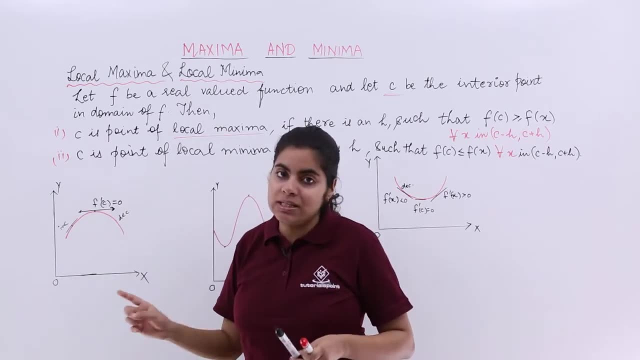 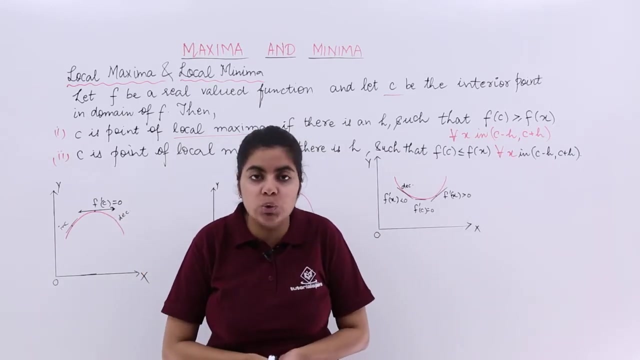 So it is decreasing, So it increases, Then it attains a peak value, Then it decreases, Since it attains a peak value. after that it changes its direction. The graph turns, So these peak value points are called as turning points also. 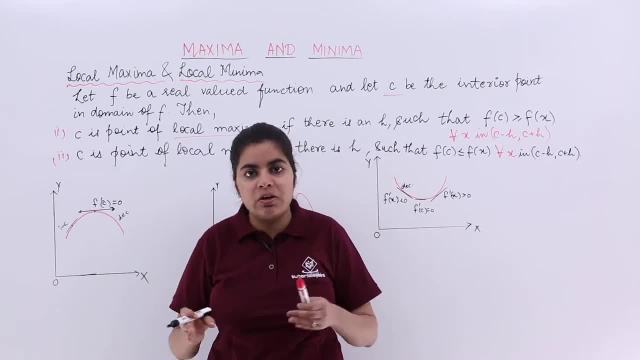 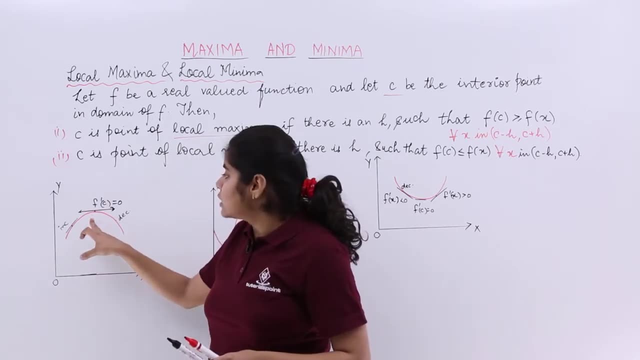 So t-u-r-n-i-n-g turning points Right. And you can see, definitely, if I have c minus h to c plus h restricted, Then this point where in my f-c becomes zero because the slope becomes such that the tangent is parallel to the x axis. 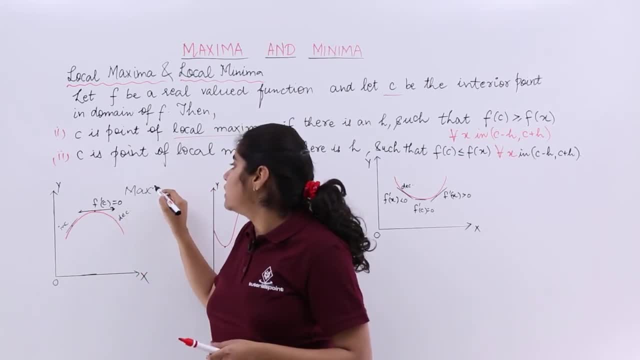 will give me the Maxima And since the domain is restricted this time, So it is not only Maxima, but a special type of Maxima called as Local Maxima. That's it. That's so simple to it. Only difference with Maxima is that the domain is restricted. 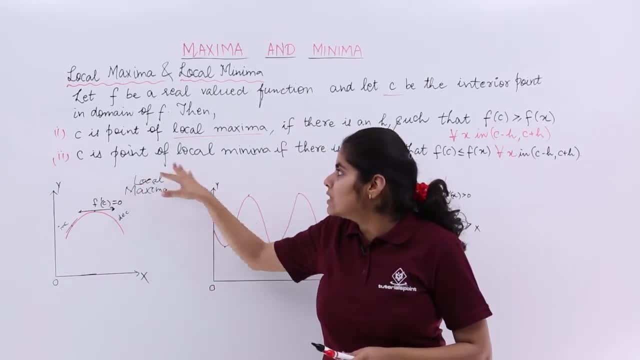 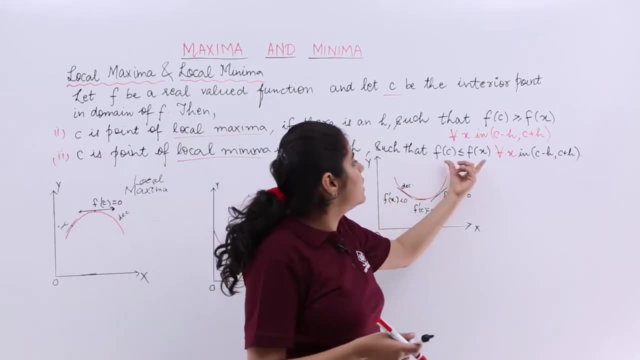 Only difference with Maxima is that the domain is restricted. is a relative maxima or a local maxima? When c is a point of local minima that we have to study with the definition, it says: if there is h greater than 0, such that f of c less than equal to f of x. 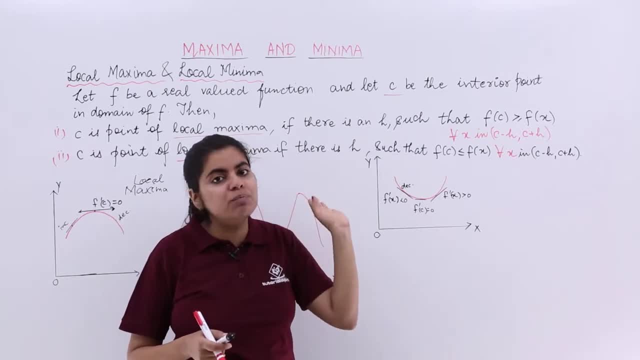 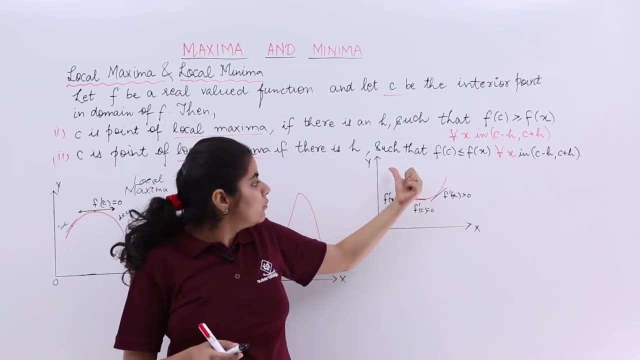 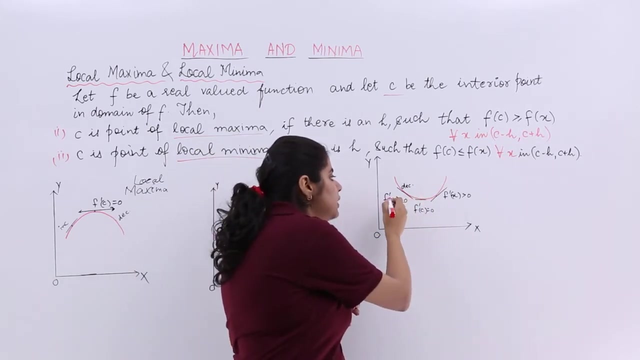 that means when c is having the value such that it will give me the least value, right, So least value would be given. So the graph would be something like this: First the graph would decrease, then you have such that it becomes such that my tangent would be there, which would be: 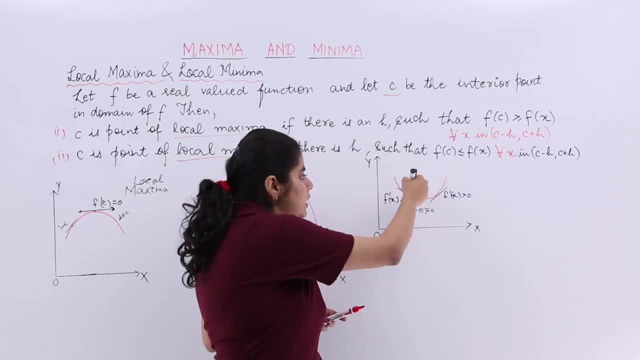 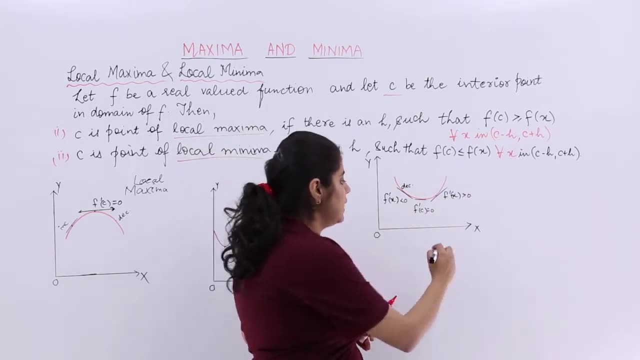 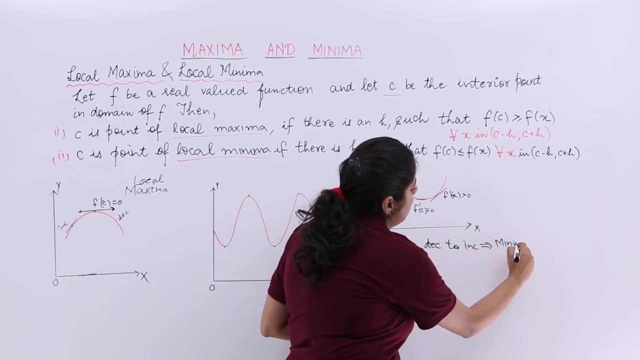 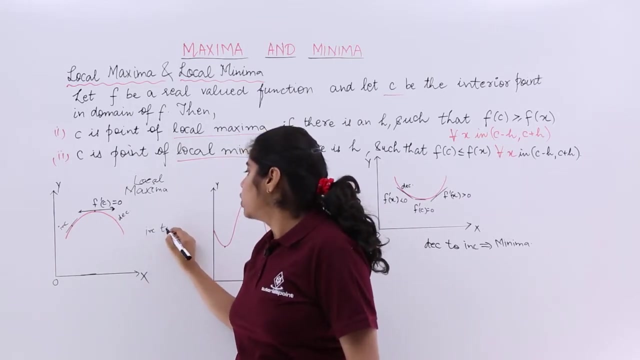 parallel to the x axis. The curve is such that first the graph is decreasing, then it is getting to a turning point and then again it is increasing. So decrease to increase, decrease to increase gives me minima, which is evident from this curve, and increase to decrease, increase to decrease. 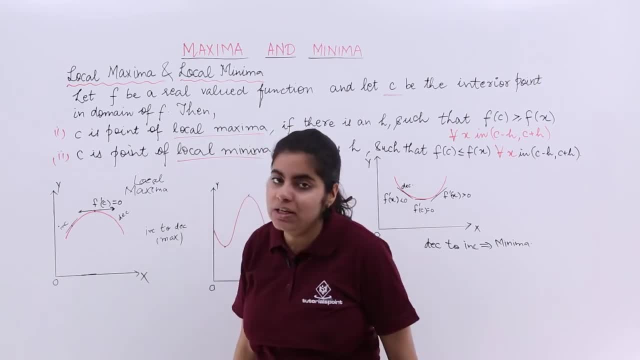 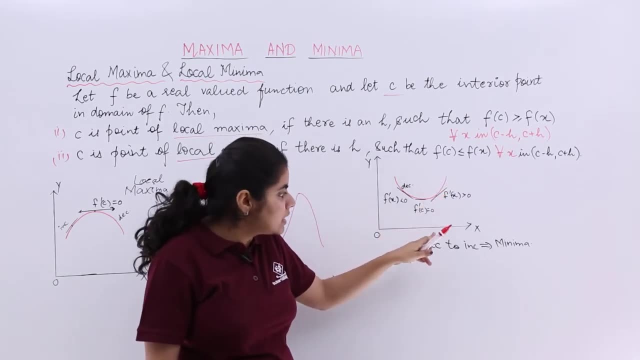 gives me maxima right. This thing we have done Now in this graph. again, if I look, if this is the point c, then I say that my c is giving me local minima, because in this domain, c minus h to c plus h, I find that my c 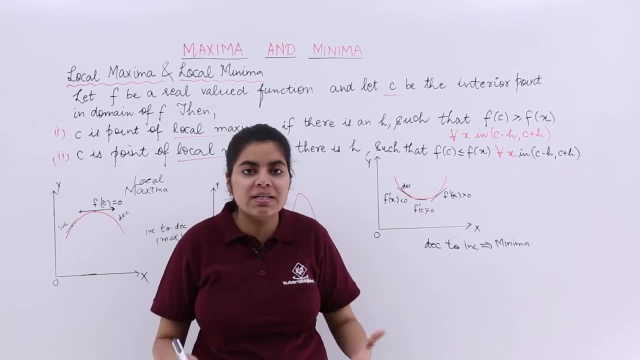 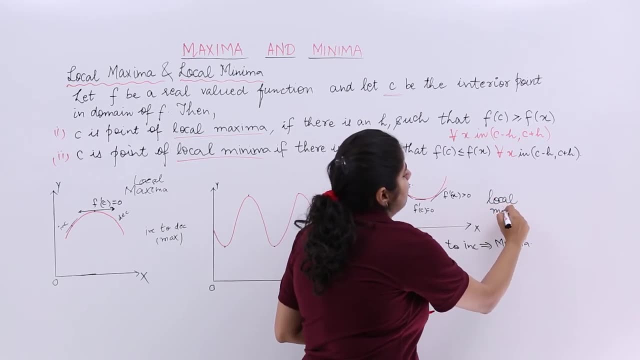 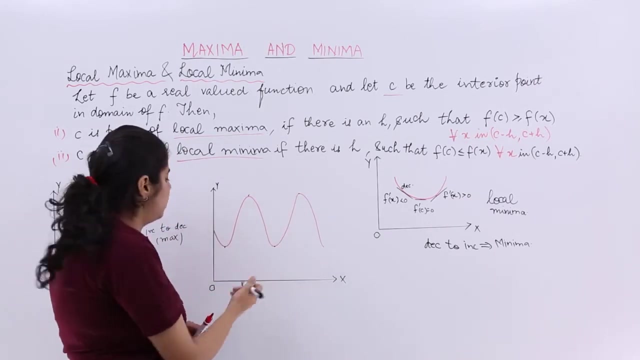 would be there, wherein f of c is less than equal to f of x, for all c minus h to c plus h. So this is local minima example. Now, if you have any random graph, say, this is the graph which is here and there are many turning points in this graph, Let's name it p, q, r, s. Let four points be. 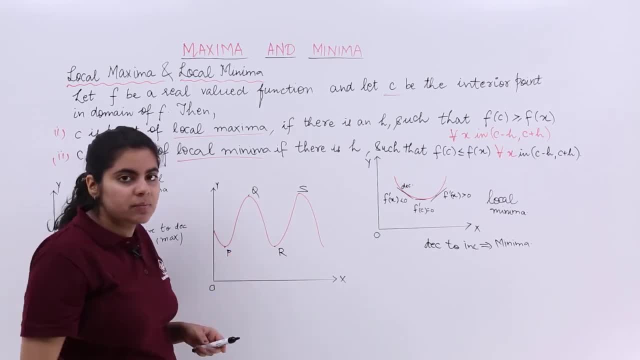 only there. Now you see that p is downwards, then the graph turns, and then q is there, which is upwards, and then again the graph turns. r is downwards. Again the graph turns, s is upwards. So that means earlier. it was what, If I have to point here, it will be decreasing. then a turning point. 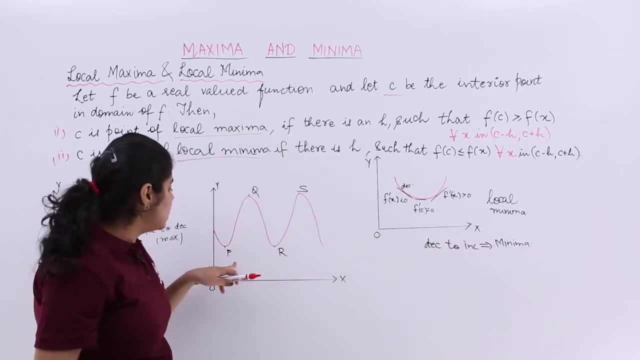 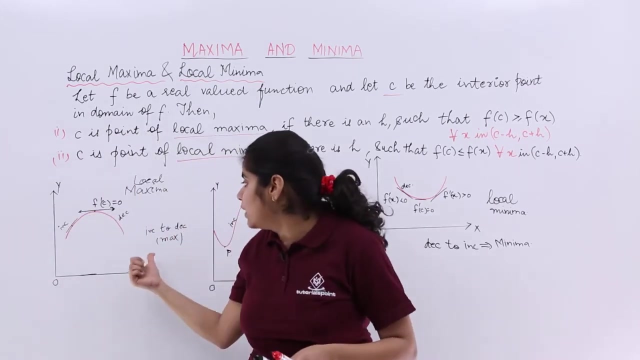 then increasing, So decreasing to increasing is minima. hence p is a point of local minima. Then again you move, so it is increasing. then it is a turning point and then it is again decreasing, So increasing to decreasing. for q, increasing to decreasing is maxima. So q is a point of local maxima. So it is local maxima. 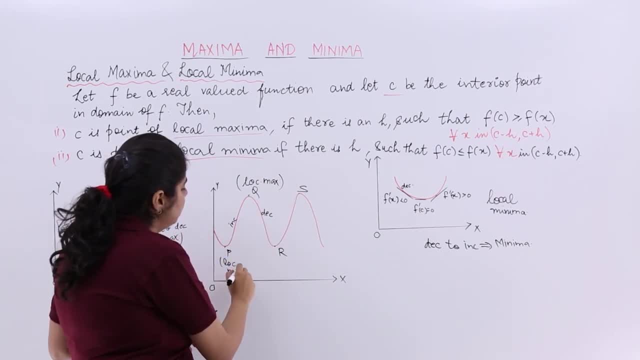 and wherein this is local minima. Now you get it, how to solve it, How to understand, with the help of graph. So we know that this is a decreasing, almost like a curve, ready to be solved. This is disagreeing. r comes and then the graph again butter. So decreasing to increasing, decreasing to increasing is minima.